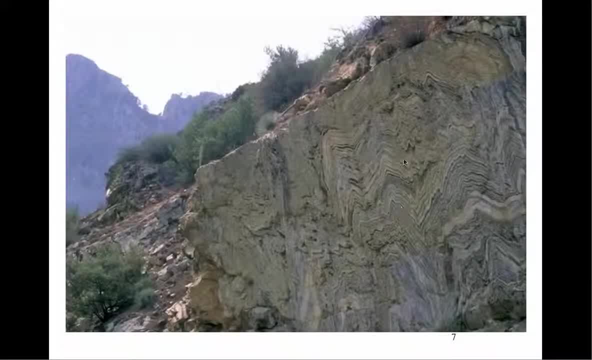 Take a look at these rocks. These rocks which probably were at one time horizontal. something has happened to them. Now imagine if you took a bunch of sheets of paper, stacked them on top of a table. What could you do to get sheets of paper to do this? 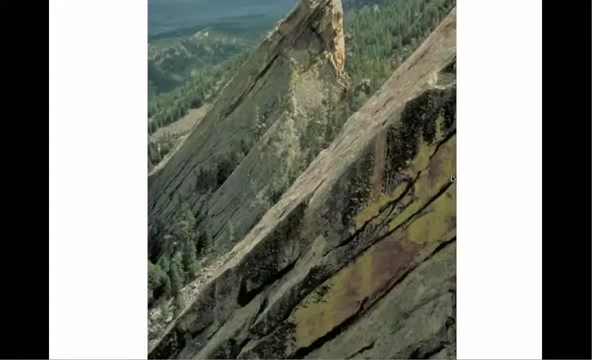 The obvious answer is: crunch them together, And that's what happens with the earth, And sometimes things are just uplifted, at least when we look at part of it. There's probably more going on to this than what we see in the picture, but that's enough for now. 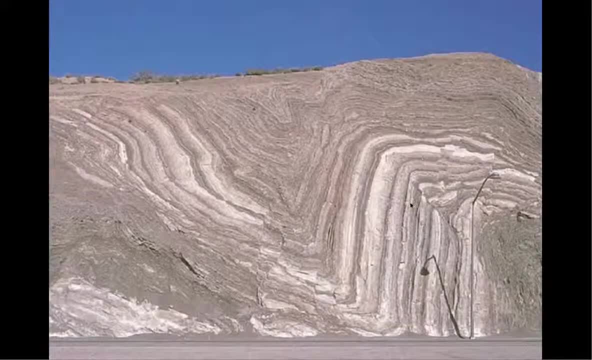 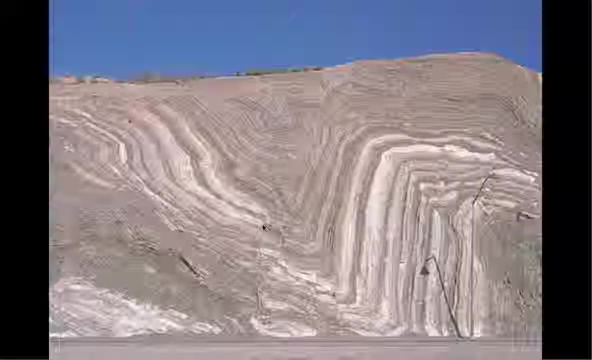 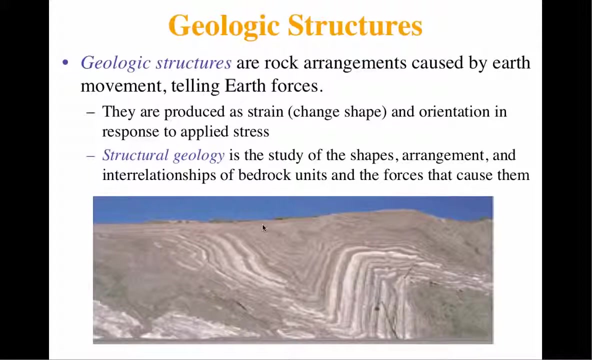 And this is just crazy. We have here some folding going on. Here's what we call an anticline, a syncline, And then it just broke here, Weird. Okay, geologic structures are rock arrangements caused by earth movement. They relate to earth forces. 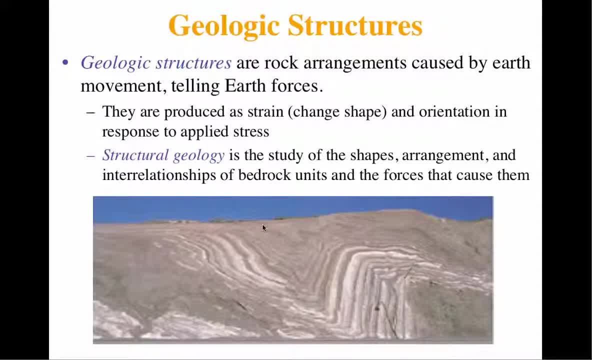 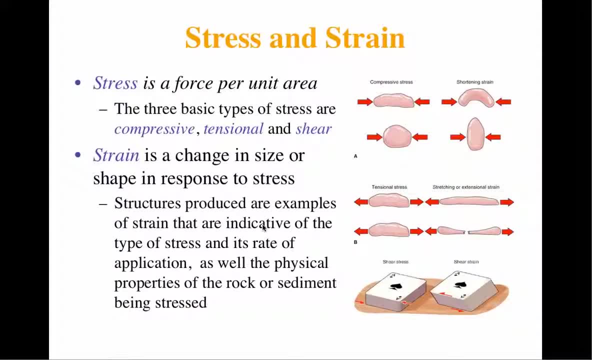 They're produced by strain. Now, a strain is anything that'll change its shape. Here are types of stress and strain. The three basic types of stress are compressive, tensional and shear. What's compressive? Squishing things together. 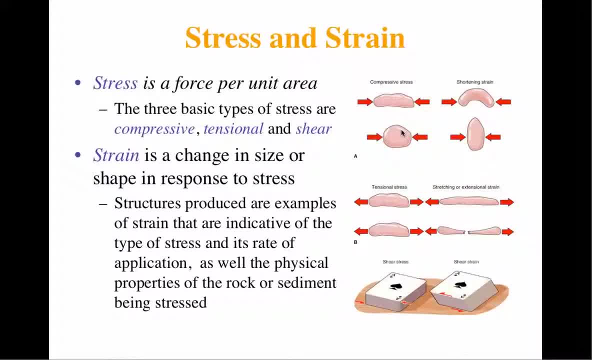 Take some silly putty and squish it. What is tension When you take the silly putty and you pull it apart? And what is shear When you take a deck of cards and kind of swipe it to the side. Now those are forces. 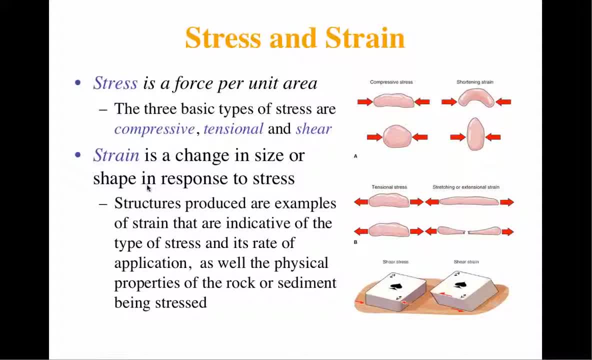 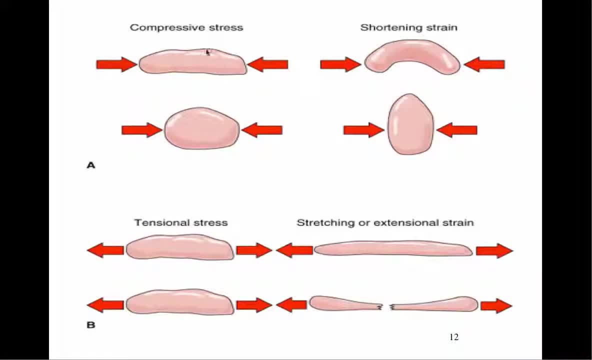 Strain is the change in size or shape in response to stress. I won't ask you a whole lot about strain, but I just wanted to put it in there Again. here's compression, and it can cause folds. Here's tension, and it can cause lengthening or breaking. 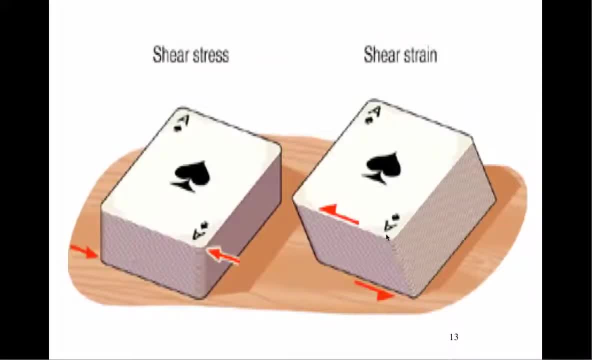 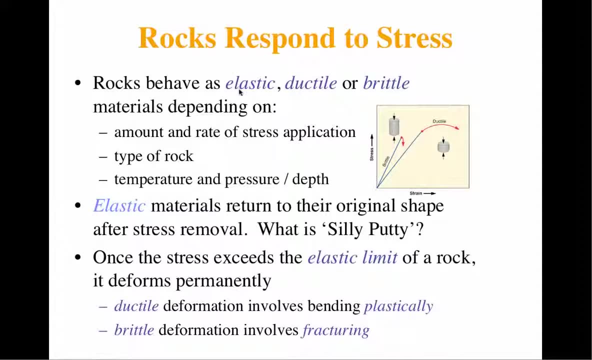 And here is shearing, and this can cause things that I'll show you in just a while. Now rocks can behave elastically, like bending, as in this kind of stuff. They can misshape or they can actually break. Now, can that really happen? Think of silly putty. 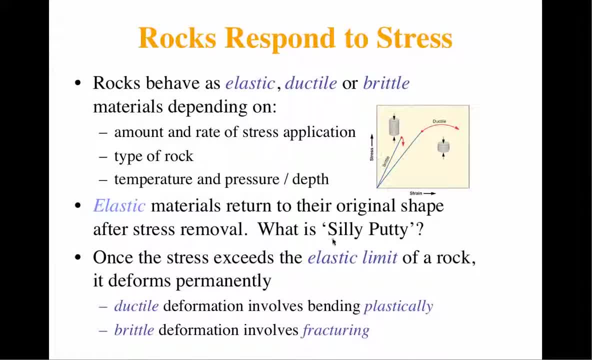 If you pull it slowly, it deforms. If you pull it quickly, it snaps. Now, elastic materials normally return to their original shape after stress removal. Think of a plastic ruler: You can bend it, but it goes back to its normal shape. 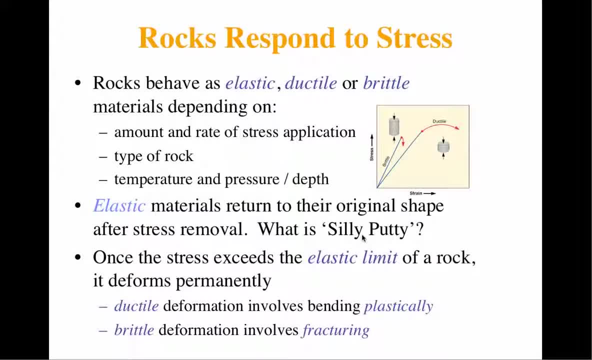 Silly putty. on the other hand, if you stretch it, does it go back to like it was? No, Now there is something called the elastic limit, Just as we were talking about with the plastic ruler. you can bend it and it'll snap back. 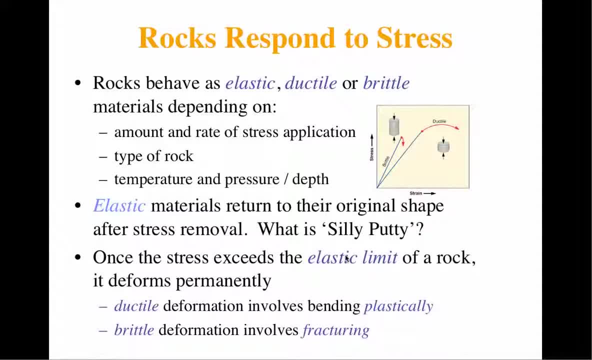 until you reach the elastic limit. After you reach the elastic limit, it may snap, meaning it fractures, or it may do what's called ductile deformation, which means it just keeps its bend. I don't think that really happens with many plastic rulers. 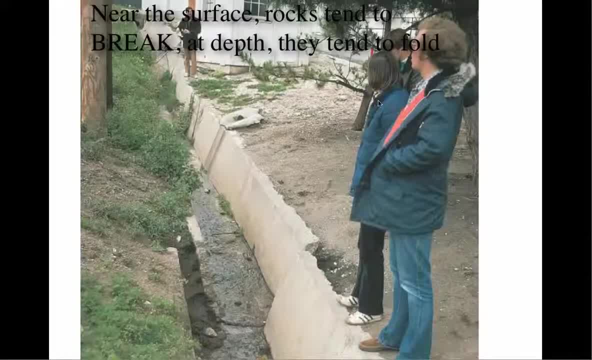 Now this is important. If rocks are near the surface, they don't tend to fold, they tend to break. Why? Because nothing is constraining their motion At depth. that's when we find rocks getting folded. These rocks, these have folds in them. 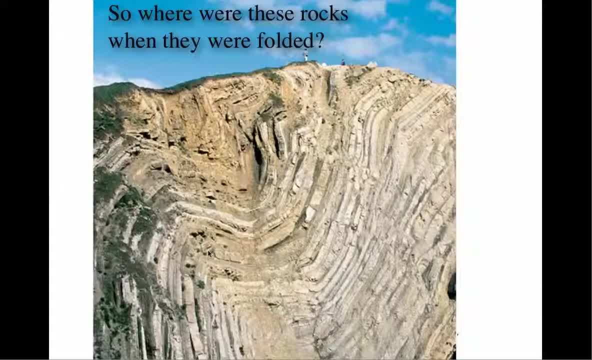 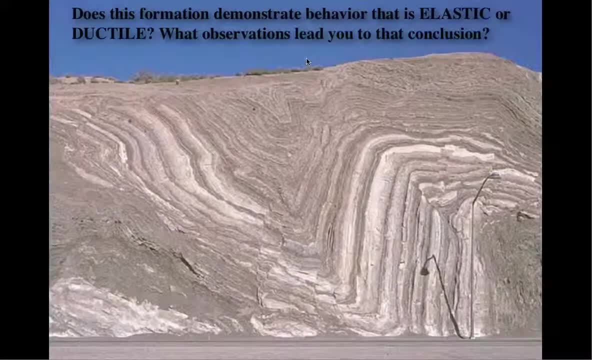 which means they were, at the time when they were formed, far underground, without these guys up here standing on them. Okay, so let's look at this: With these rocks near the surface or far underground folding, which means it must have been far underground. 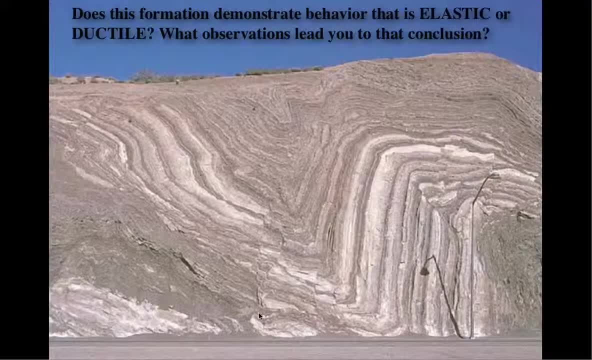 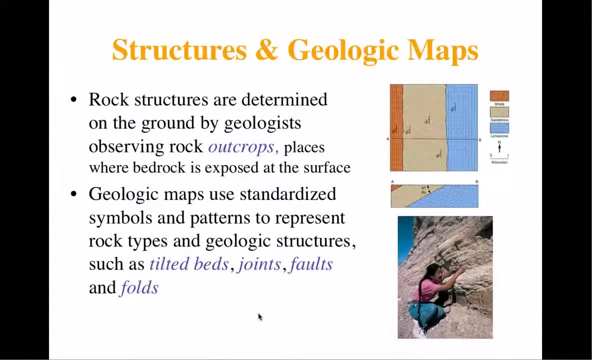 and then we have faulting, which tends to happen more close to the surface but not always on the surface. Now an important Have I said now a few times in here: Aw, gross Geologists love things that are called outcrops. 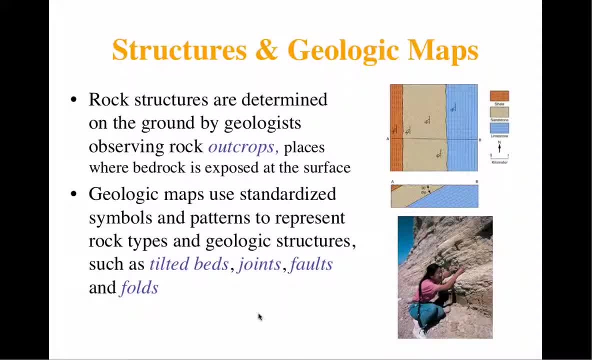 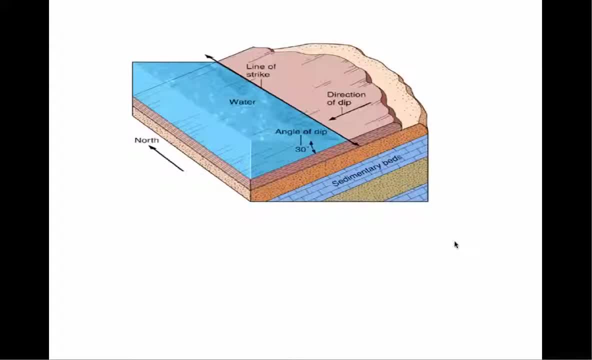 These are any areas where rocks are exposed to the surface. This is an outcrop. Now, in the movie that you're going to watch, you're going to learn about this. This is called the strike. This is called the dip. The direction of the strike in this case is north. 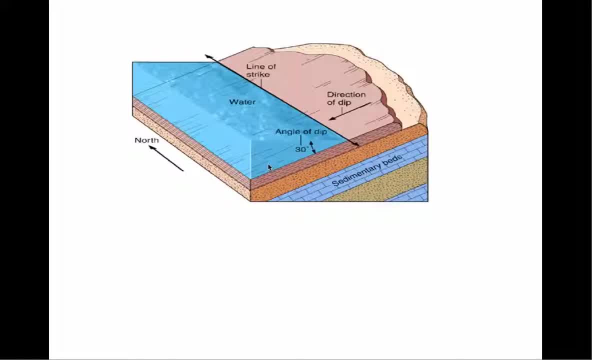 and the angle of the dip is 30 degrees. In a real earth science class you'll be looking at geologic maps and messing with this kind of stuff, but we're not going to do it here. What do you use to do that kind of thing? 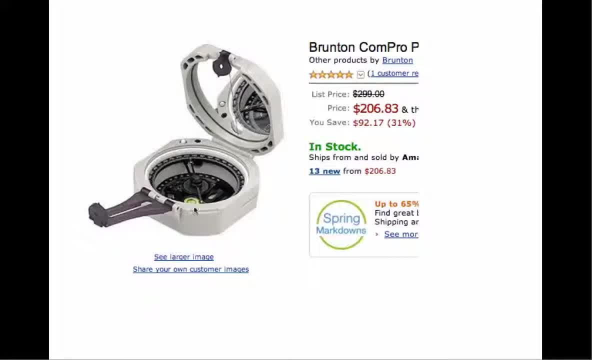 The movie talks about one kind of instrument. This is the more common kind of instrument. This is a Brunton compass, and you can buy one of these for only $206.83.. This was off eBay, No Amazon, I'm sorry. 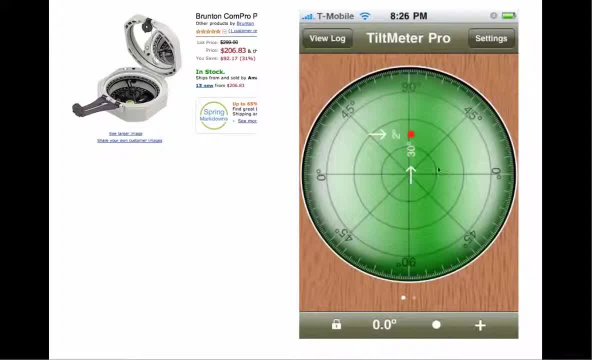 What's kind of crazy is. you can get the Tiltmeter Pro, I think, for $0.99 on your iPhone or other Android phone. This will do the same thing. I don't know. I just think it's kind of cool what's happening with smartphones. 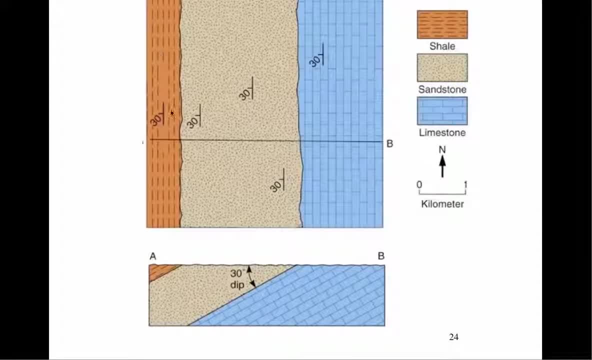 Now, what's going on here? This is a geologic map. What are all these little T's? They're showing you that the rocks are dipping down into the earth at an angle of about 30 degrees. In this case, the strike is going north. 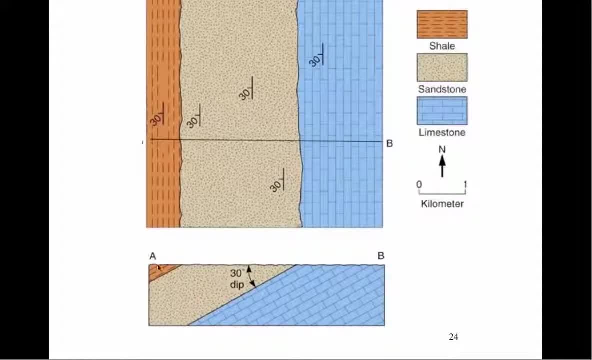 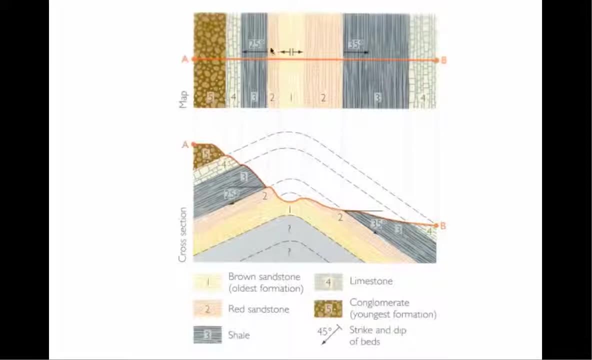 If you were to walk along here, you'd be going across sandstone and then across limestone. Ah, we have a key over here That'll be handy. Here's a slightly more complicated thing. Here we have dips going that way at 25 degrees. 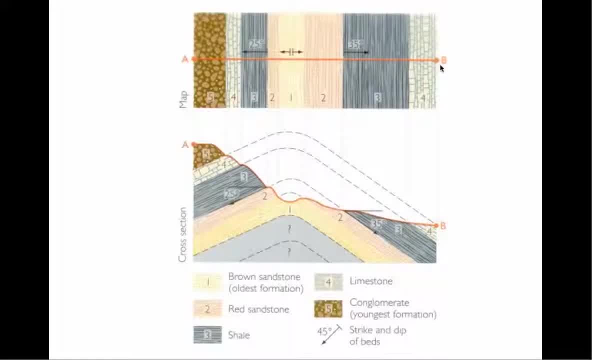 We have dips going this way at 35 degrees and you have several different types of dips. You've got shale, which is the number three. Two is a red sandstone. One is a brown sandstone. Limestone is typically the brick formation and conglomerate here. 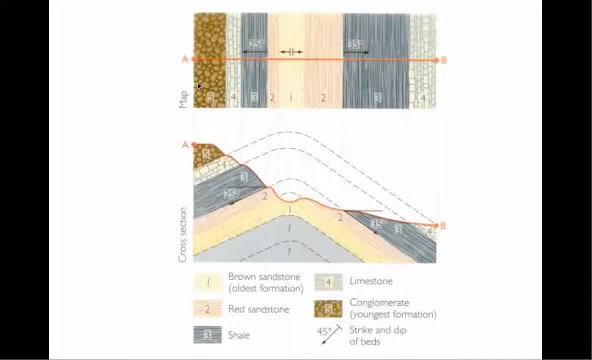 These are slightly different drawings than normal, But if you were to draw this in cross-section, this is what you'd be seeing. This is called an anticline fold. It looks like the letter A for anticline. The rocks have been squished together. 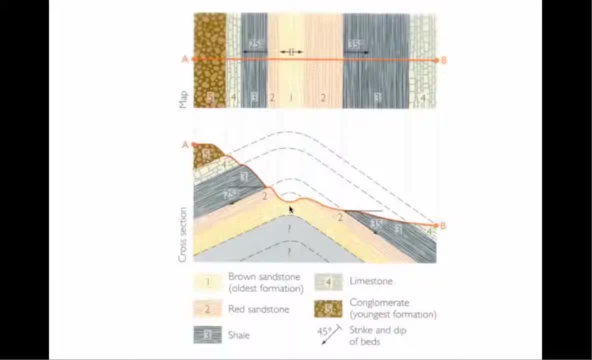 and this layer that's in the middle is the oldest layer. What's happened? This was bent up and then down, and because this was bent up and down, it gets really weak in this area If you've ever taken silly putty and bent it like this. 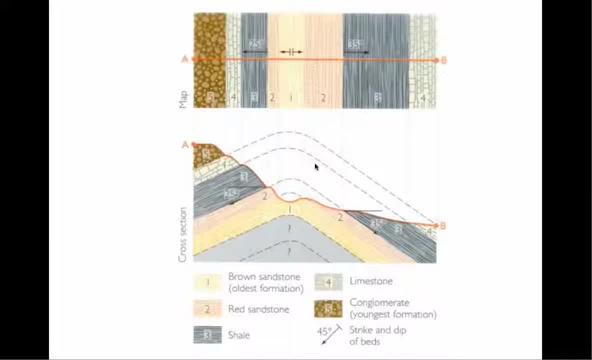 you know that you get cracks right along here. In the same way that a glacier going over a ridge will create crevasses, this creates cracks and these cracks tend to wear down really quickly. Okay, let's look at this outcrop. 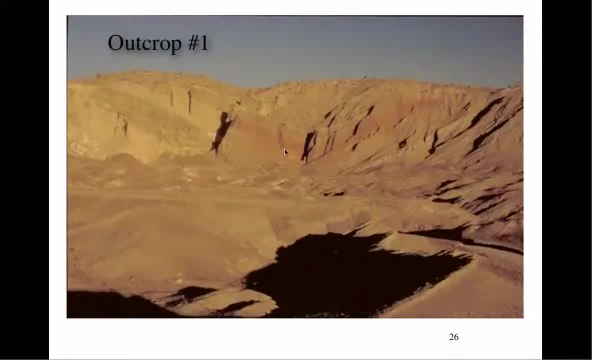 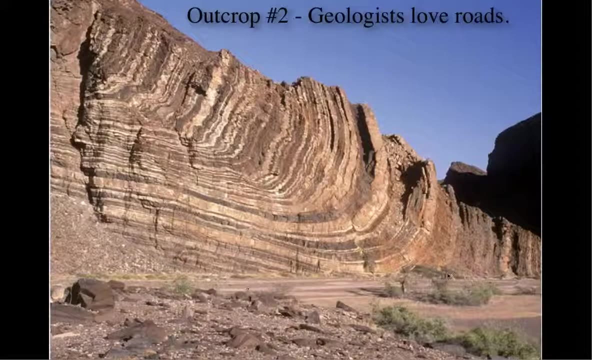 What's going on here? We've got folding, but instead of being up like this one, it goes down. This is called a syncline. Here is an anticline along a road cut- and geologists really do like roads, because they expose a lot of rocks that we can look at. 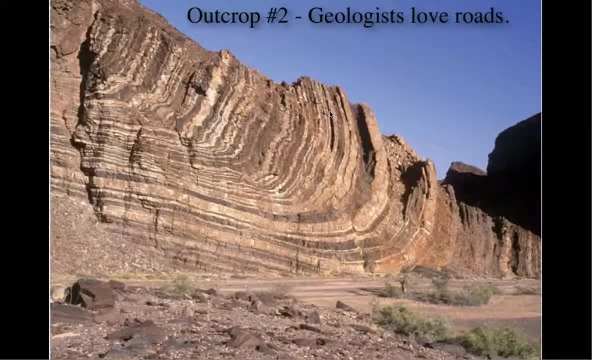 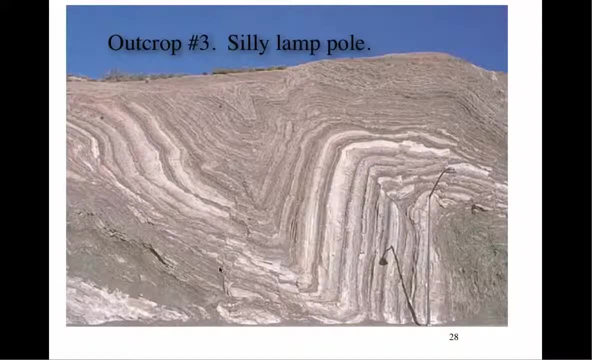 These are old sedimentary rocks that by now may be metamorphic due to all the pressure. And again, here you have an anticline and a syncline and a fault all in one. Now this goes into a little bit more depth than we really want to do. 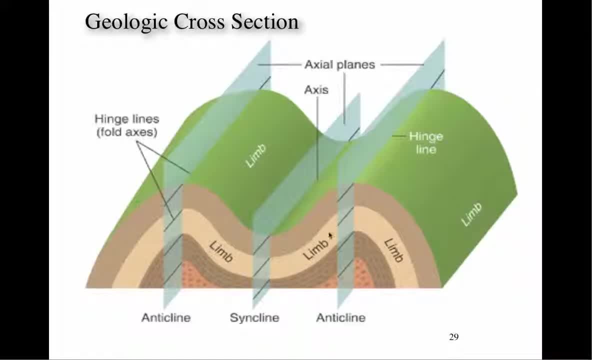 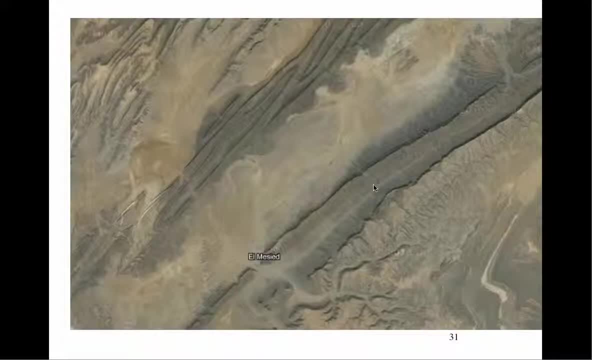 but here again is the anticline, Here's the syncline. That's good enough for now. Now, types of structures. This is out of, I believe, either Molly or Chad. I got this off of Google Maps. What are we looking at here? 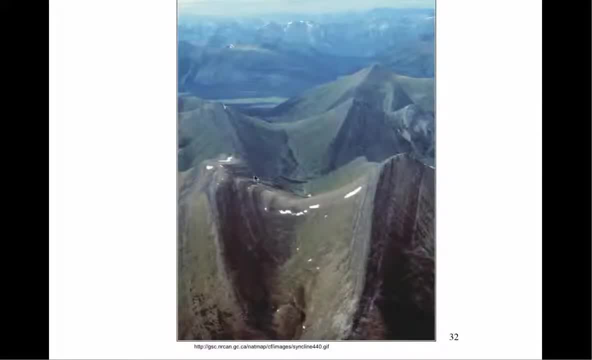 This is a satellite view, looking straight down at something kind of like this: This area is from the northern Rockies, where rocks have been folded up and back down. Boy, take it back. This is a syncline. This is kind of crazy. 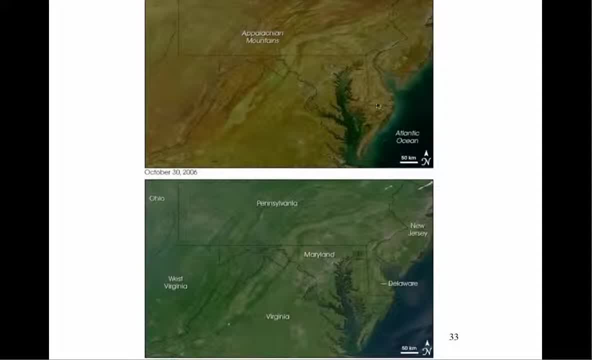 Here we are in the Appalachian Mountains, where North America has run into Africa, and all the rocks in here have been squished together just like a towel on your tabletop. If you squish it together from left and right, it's going to get all these wrinkles in it. 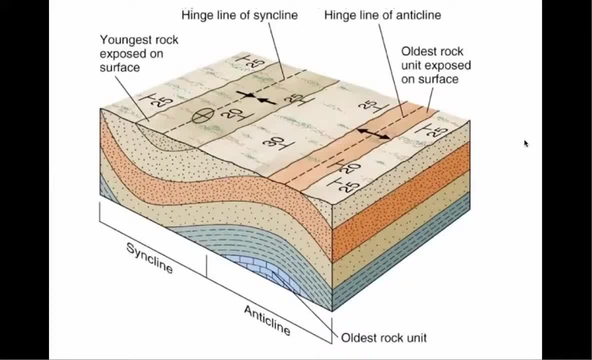 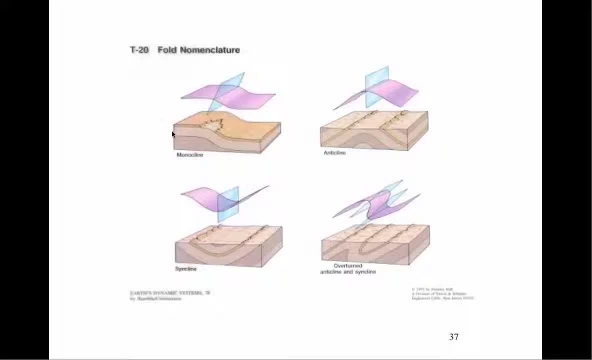 Folds Again. this is a little bit more technical than we want to go, but let me cover a few things. A monocline is when you just have one bend Again. where you get bending, you get a lot of erosion going on. 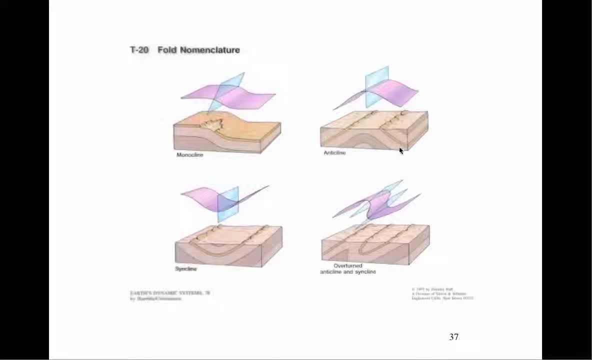 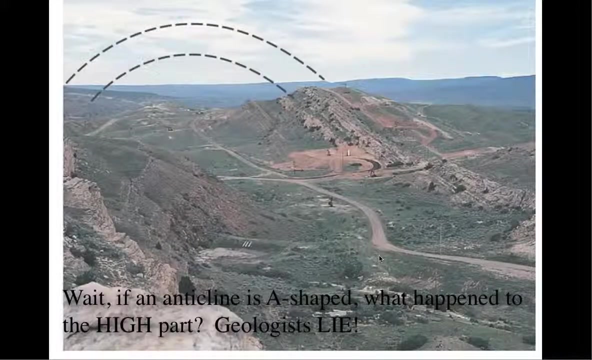 An anticline is where you have an upward fold in the middle. A syncline is where you have a downward fold in the middle. This is just a mess. These are overturned anticlines and synclines. Now, once again, the highest part of an anticline. 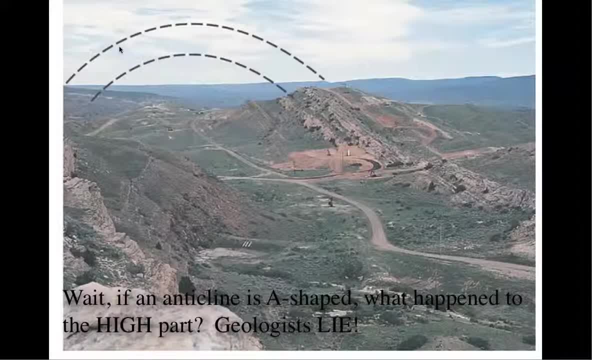 tends to crack and it gets worn away first. This is a little bit weird. This is a little valley in Colorado where they are beginning to fracture for natural gas and go in for oil, and the water, for some reason, is not very good anymore. 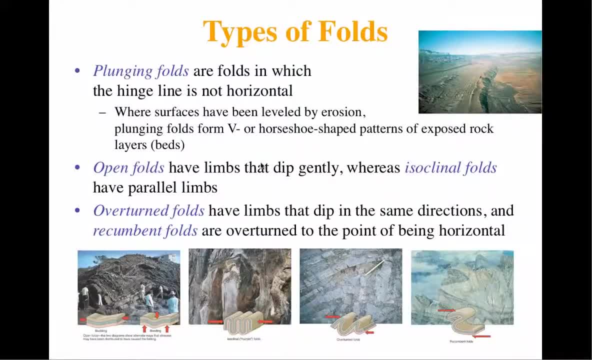 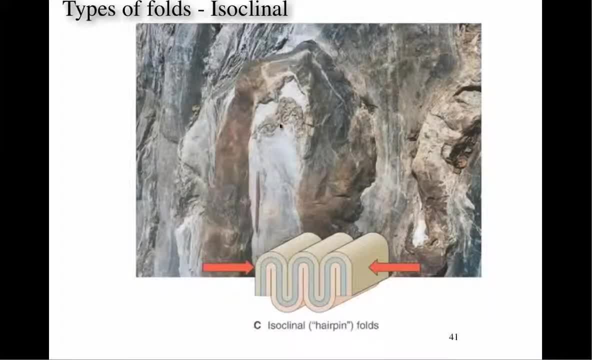 Now a little bit more on folds You can get. Well, let's go into the big pictures. You can get these crazy folds. These are called isoclino folds, but I don't want you to memorize that It's not a big deal. 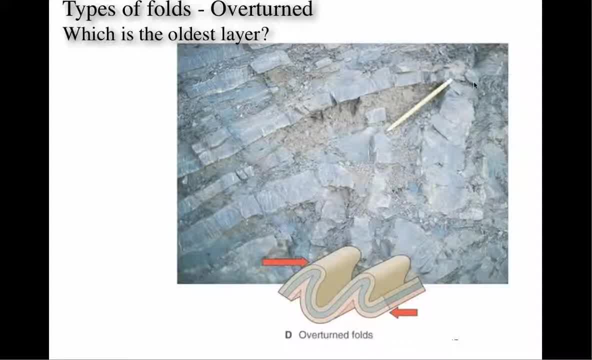 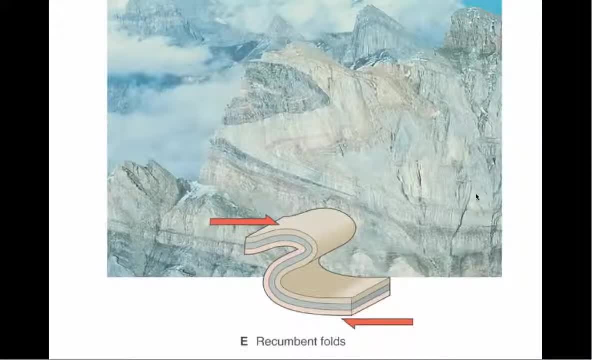 You have overturned folds here. The pencil is there just for size reference. And in the Ura Mountains in Switzerland, you have recumbent folds where rocks are folded back on themselves. Again, this doesn't happen at the surface, This happens only at depth. 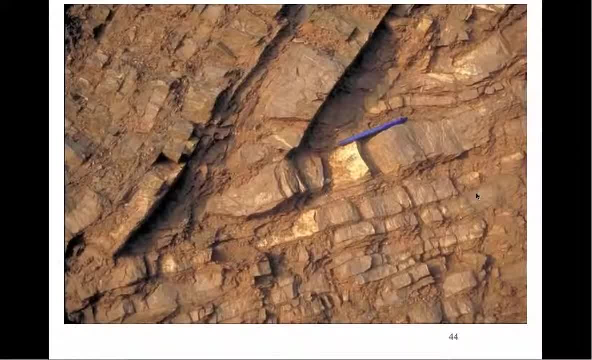 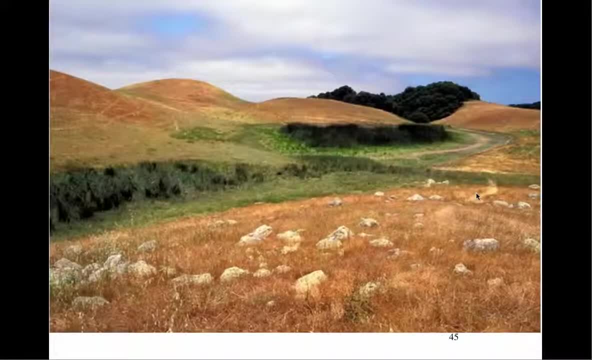 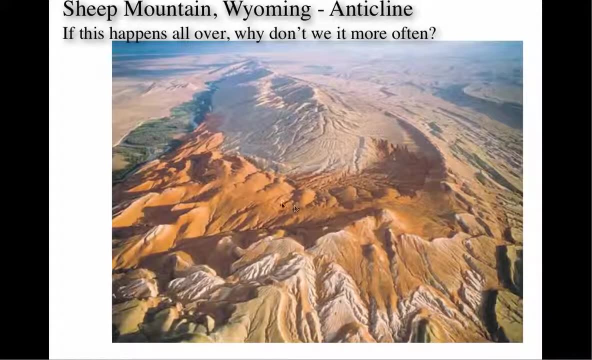 and it takes millions of years for this to occur. Take a look: Big recumbent fold, small recumbent fold, And there's just a pretty picture. Let's relax for a minute. Okay, let's keep going. Anticline. 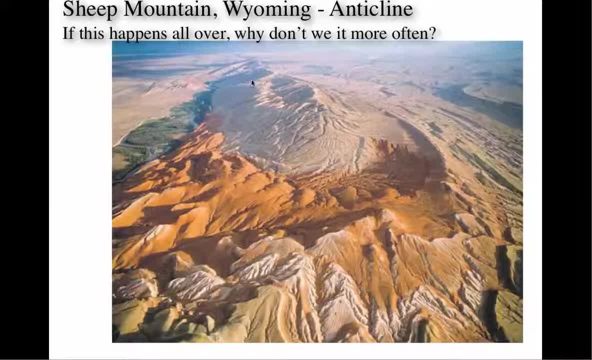 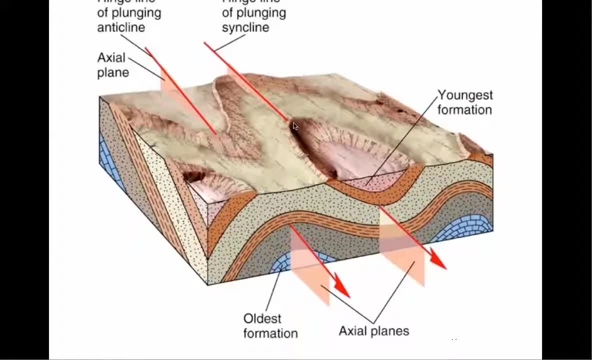 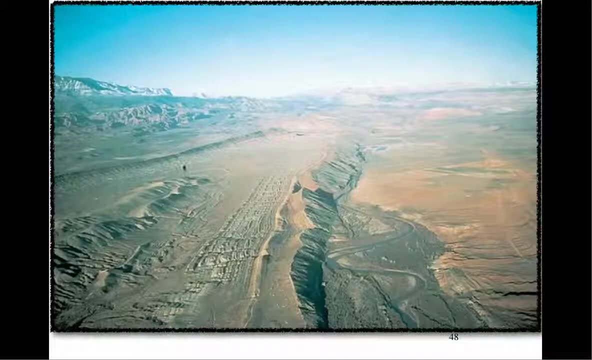 This is in Wyoming. This is Sheep Mountain, Kind of a beautiful area. Why don't we see anticlines more often? Here's an anticline I forget. I think it's Sheep Mountain again. We're just looking in the opposite direction. 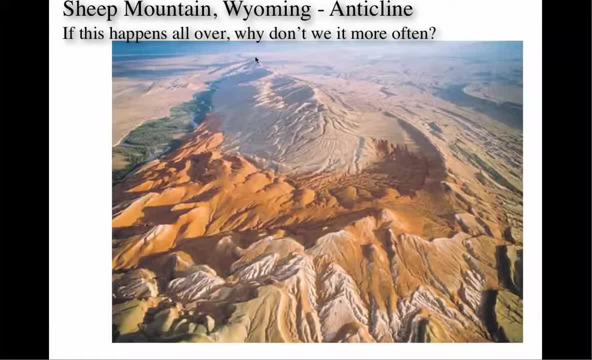 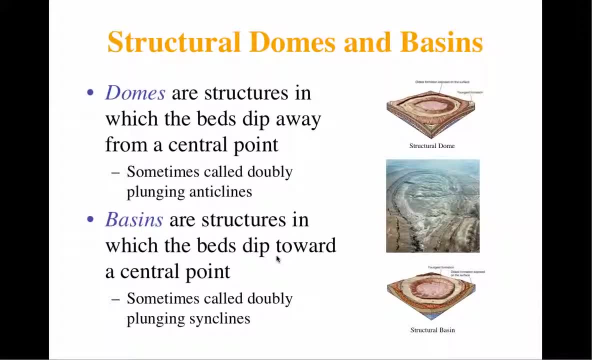 Take a look, There you go. In this case, we're looking from the north. Now, one of the things that helps create anticlines are domes. If you have something underneath a towel on your table and it rises up, let's say you put your dog under there. 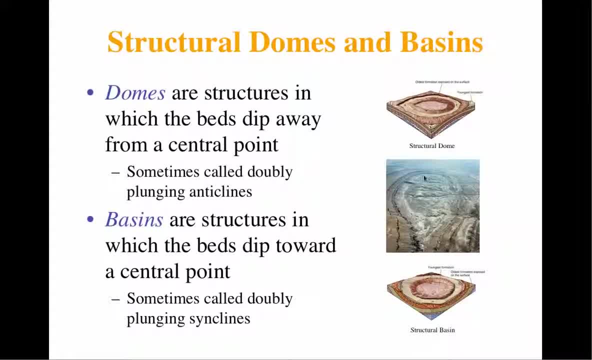 and your dog stands up. you're going to create a dome out of the towel And that can form an anticline. It's called a structural dome. You can also get a basin which is kind of like an antidome. Here is a dome. 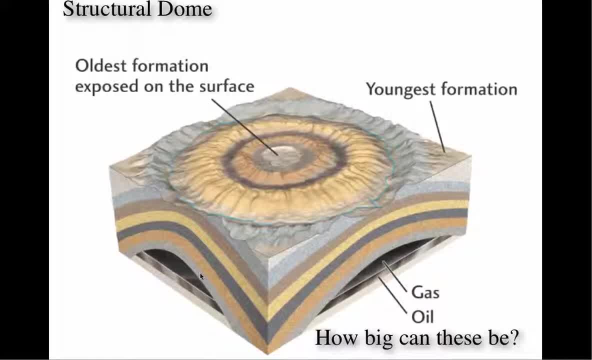 And in this case- In this case typically, these are caused by a really low density of material underneath, causing the sedimentary layers on top to arch over. You end up with these really weird erosion rings and you can look underneath this- for gas on top, oil on the bottom and water underneath. 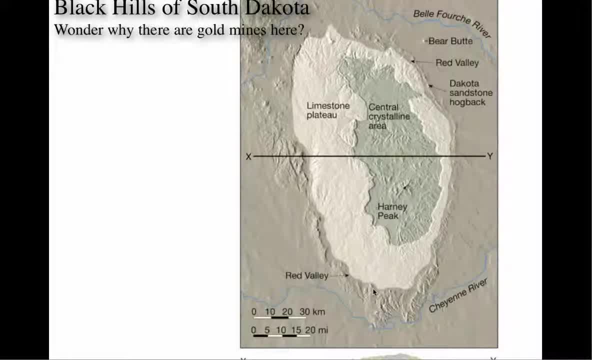 Here's how big one structural dome can be. In the case of this dome, it appears to be about, I would say, about 40 miles across and about 70 miles from top to bottom. These are the Black Hills in South Dakota. Here is another dome.